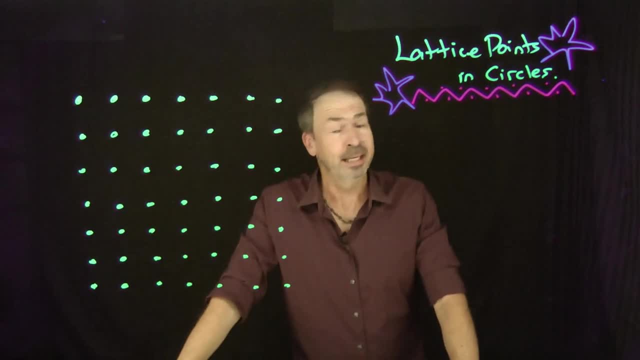 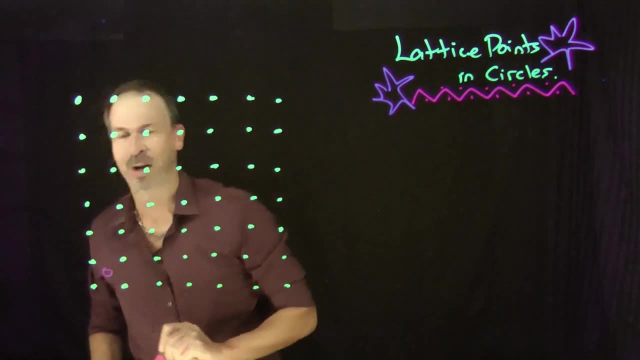 avoid going through lattice points, but I want my circles to actually contain on the interior some. For example, I could draw a circle that contains zero lattice points. A little tiny circle like that would do the trick: No lattice points on its inside. I. 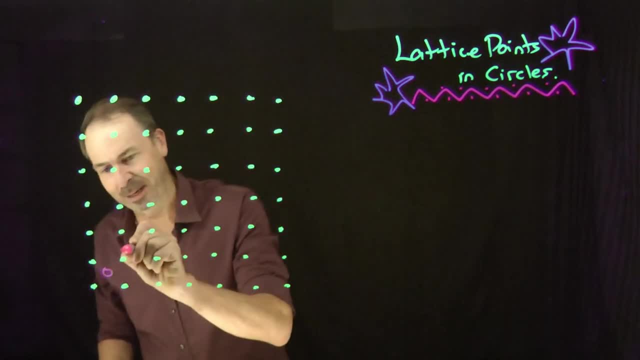 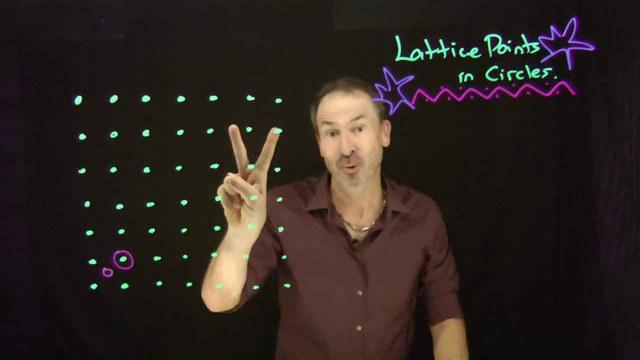 could also draw a circle that contains exactly one lattice point, Namely something like that, would do the trick, But then I want to keep going. Could I draw a circle that misses all the lattice points itself, but contains exactly two lattice points on its inside? 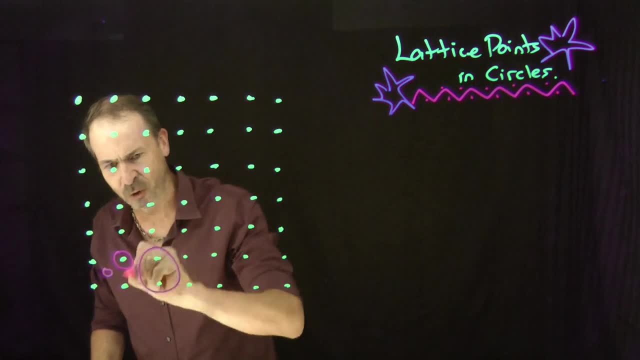 And you think for a while that maybe I could set things up so a circle like that would actually do the trick. My picture's a bit wonky, but maybe that's believable. I could actually do that. You could check on that one. Could I draw a circle like that that? 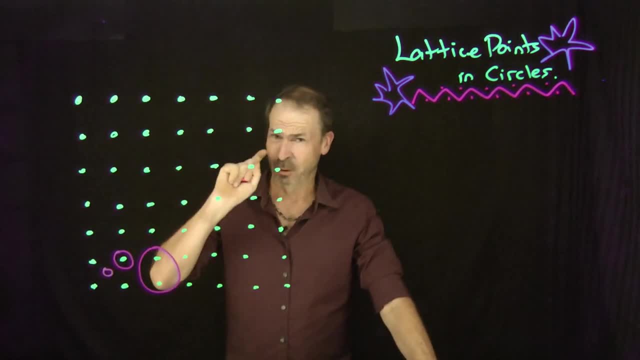 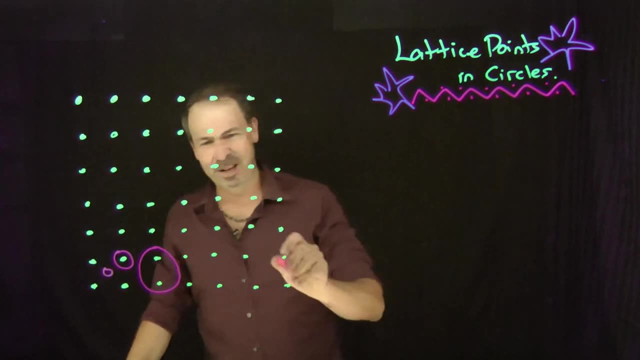 really does it. Three lattice points on the inside, Remember, I want my circles to miss going through lattice points themselves. but I want now three lattice points on the inside. Do you think that's doable? And you stare at it a while and you think, well, maybe it's possible to get a circle like this. Oh looks. 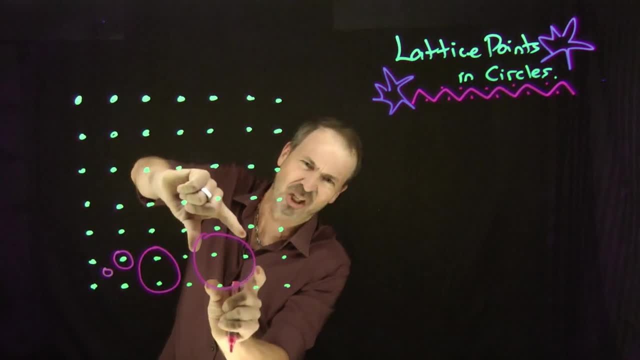 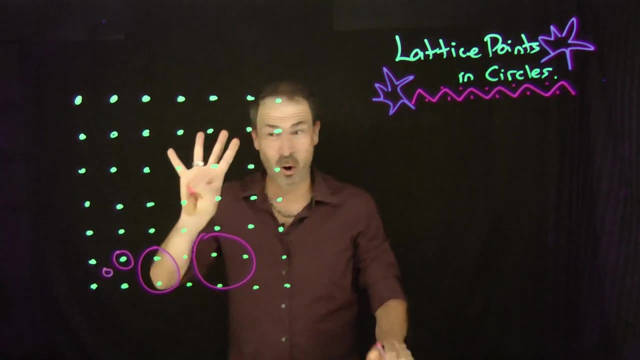 like I just hit that one but maybe miss it. Maybe there's one that can be arranged just like that that just misses it. Is that possible? Ooh, ooh, my pictures are not very good, Hard to tell. Okay, but I'll keep going. Four lattice points on the inside. Well, that feels believable. 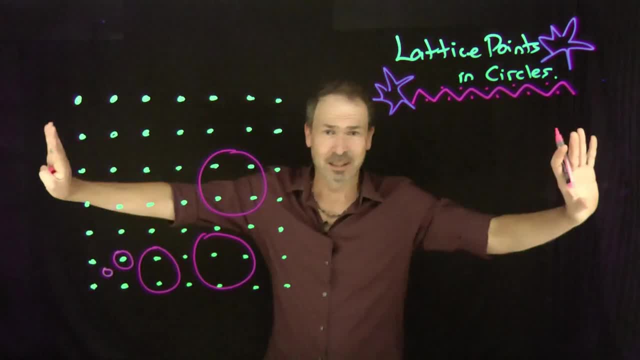 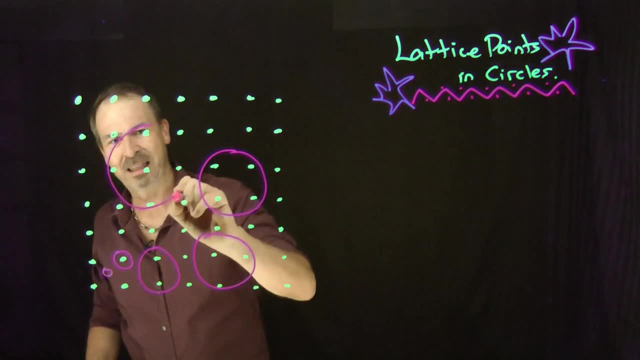 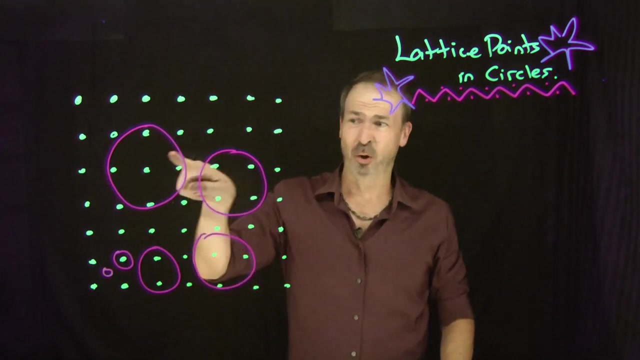 Maybe I could do something like that. Five, A circle that misses lattice points itself. maybe that's doable if I think of something like this. Maybe a circle like that will do the trick. Six, seven, whoa, All right. so some of these pictures here are a bit questionable. 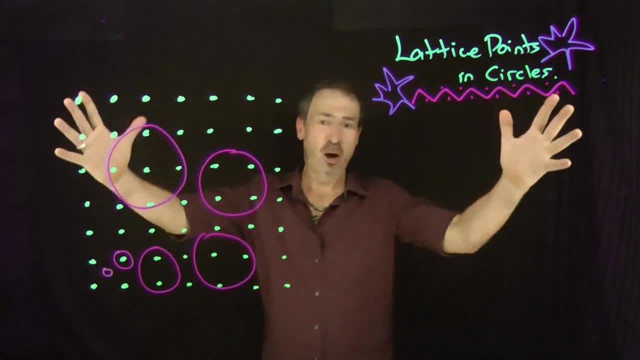 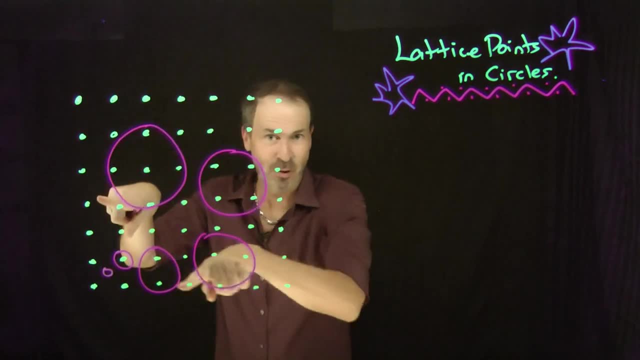 already. My question is: can it be done If I give you some count of lattice points? I want 73.. Is it possible for sure to draw a circle in the plane that itself misses going through lattice points? I don't want to go through a lattice point, but I want 73 lattice. 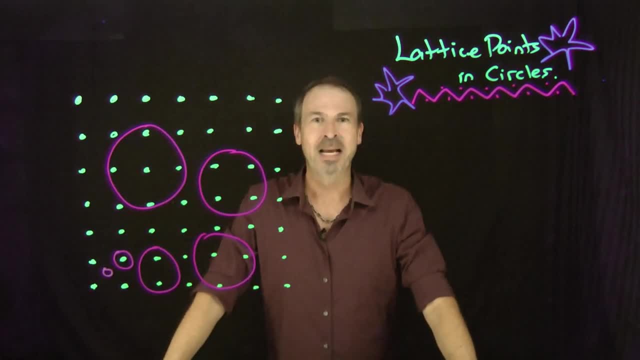 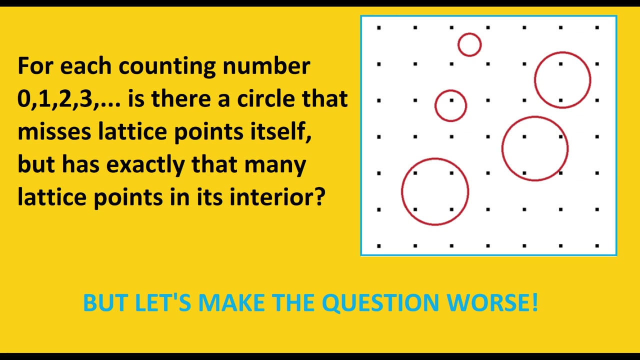 points to be on its inside. Whatever counting number I give you, is there sure to exist a circle with that number, A circle with that many lattice points on its inside and none on the boundary? That's a tough question, Actually. let's make the question worse. Could I do that and have all? 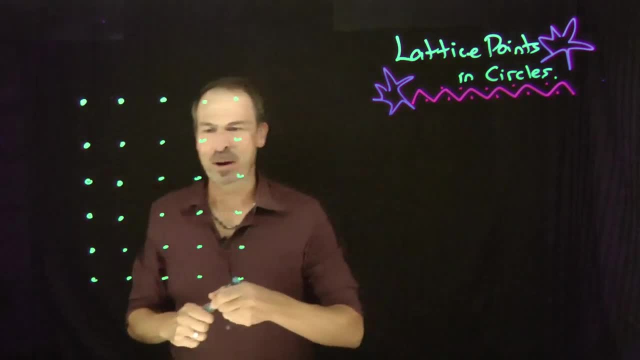 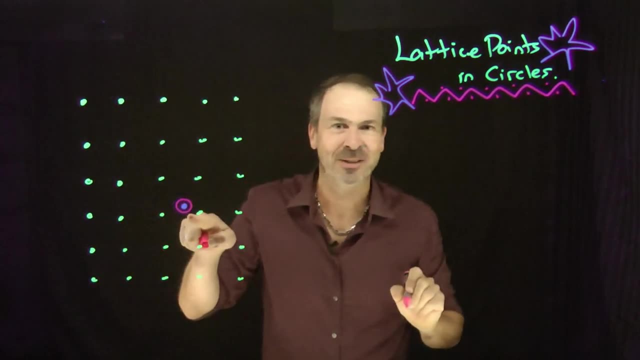 my circles be concentric, That is, I want to find a special place in the plane, maybe something like this, With a property that if I draw a little circle around it, sure I get that, with no lattice points on its inside. Make the circle a bit bigger. I get one lattice point on its inside. 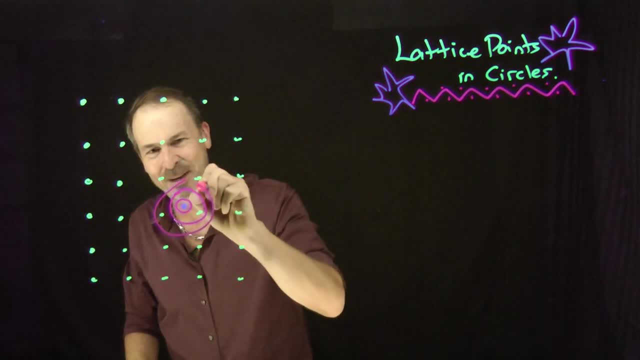 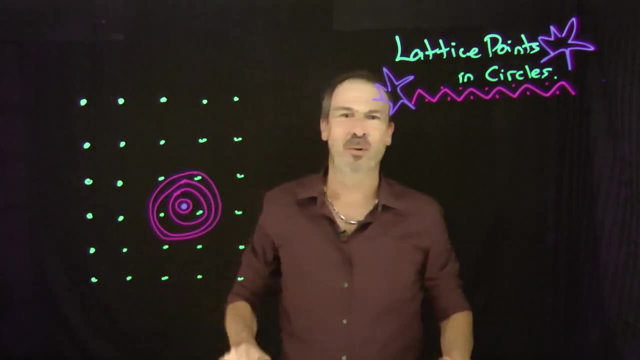 Make the circle a bit bigger still. oh, my picture's gonna be really bad here, but two lattice points on its inside Make the circle a bit bigger still, all centred about that same one point. three lattice points, four lattice points, and so on. Could there be a? 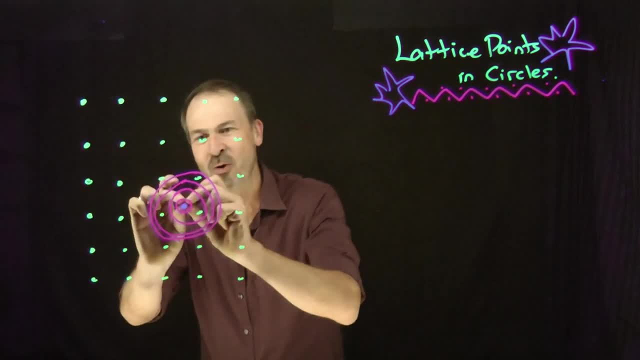 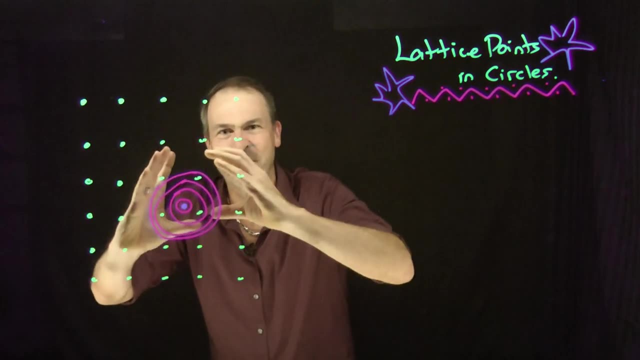 very special point in the plane with the property that could grow circles from that special point, all concentric circles that hit 1, 2, 3, 4, 5 lattice points at a time, because if I hit one up to 5 and 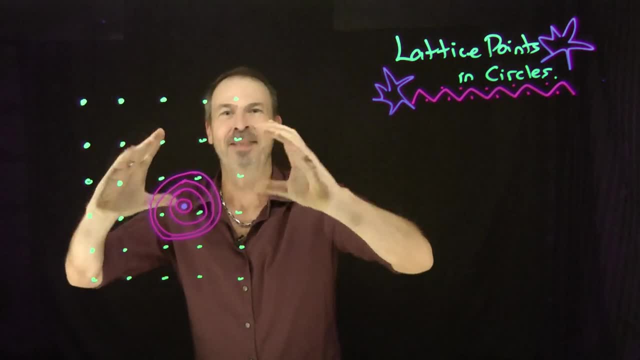 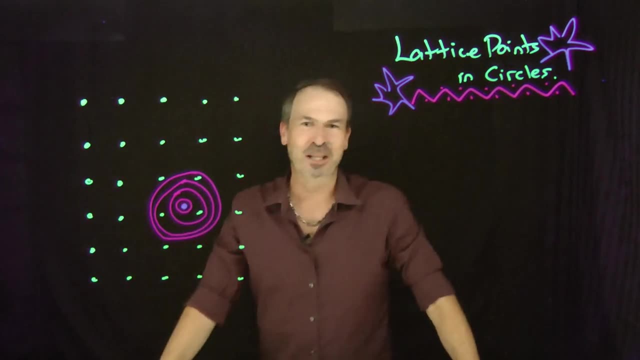 go a little bit bigger, then it will contain 5.. Hit number 6, go a little bit bigger- then it will contain 6 lattice points. Go to number 7, hit it, go a little bit slightly bigger, then it will contain 7 lattice points. Is there a special point in the plane with that? 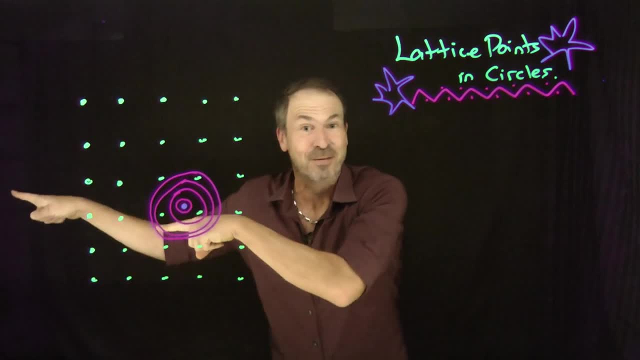 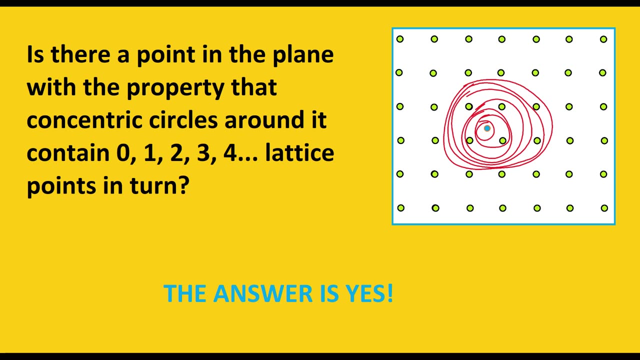 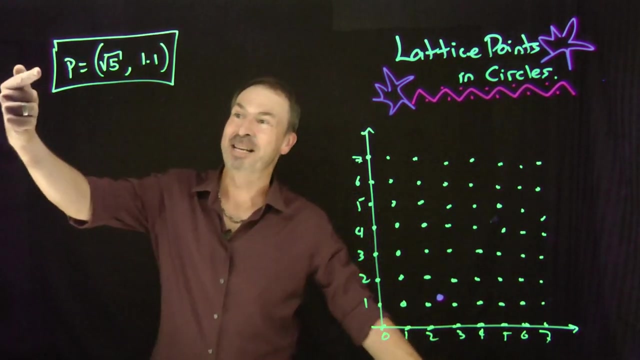 magic property, Because that would be awesome and also answers my previous question. The answer to the previous question is yes. There are such magic points in the plane. For example, this point here with x-coordinate root 5, y-coordinate 1.1, has the astounding 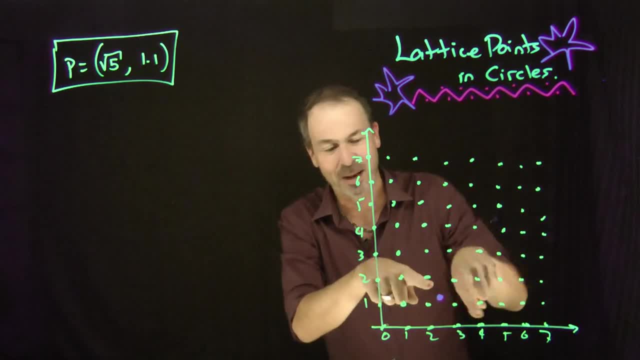 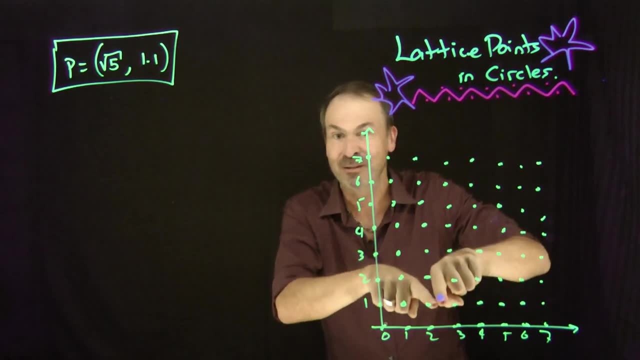 property that all the distances, the different lattice points in the plane, no matter where you go, how far out they're all going to be different numbers. There won't be two lattice points at the same distance from this one. That means then, as I expand circles, 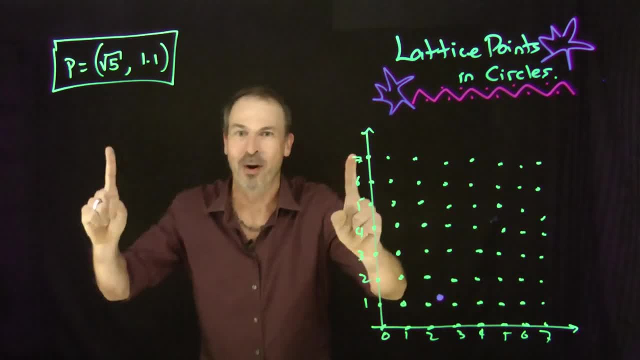 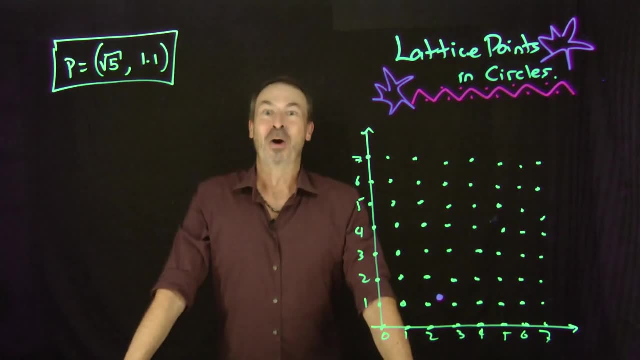 hit two points at the same time. I'll only ever hit one point at a time, just as I needed for the previous question, And I claim that is one such special point, Whoa. So I want to prove that. I want to prove that this point here, all the distances of. 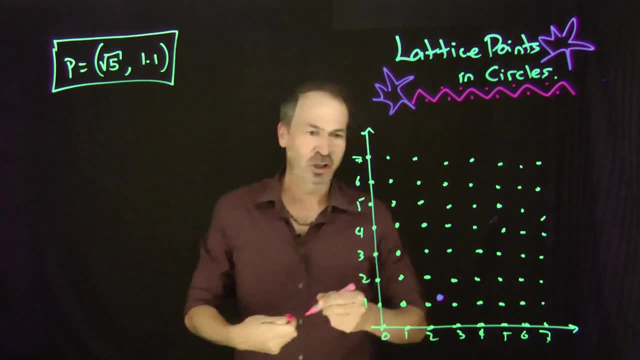 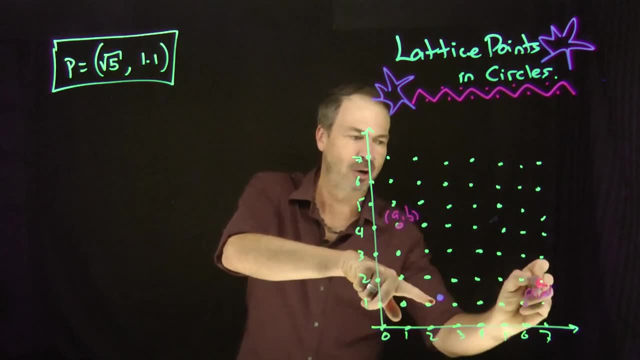 different lattice points are indeed different. You'll never be in a situation like this. where, say, this point here with coordinates a, b, both integers, and maybe this point over here with coordinates c, d, both integers, has that distance there? 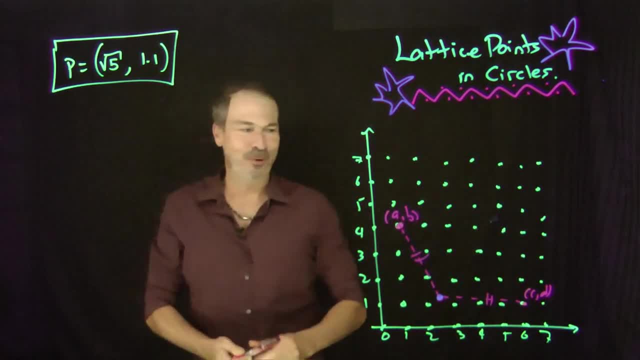 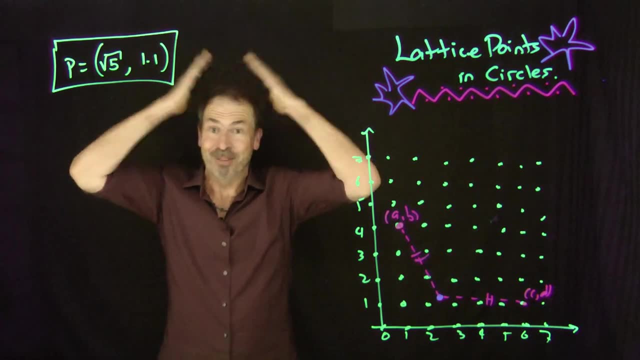 Equalling that distance there. How can we prove that never happens? All right, Well, we'll do it as follows. I'm going to do it, I'm going to use, I'm going to use basically, I guess, the distance formula, because I want to talk about this distance. 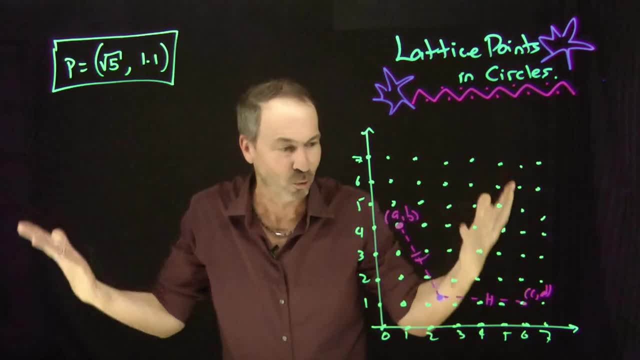 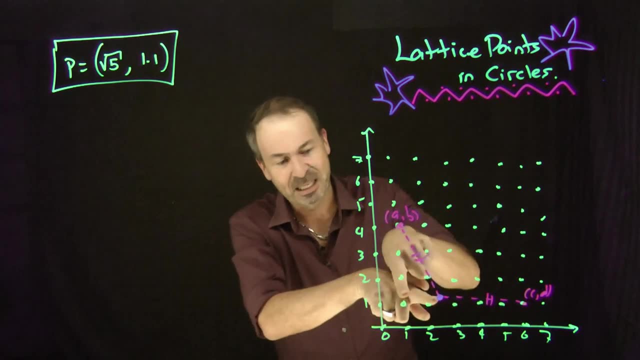 here and that distance here. Let me compare distances with the standard school geometry distance formula. What is the distance formula? Well, here's the lovely thing about using coordinate systems that are at 90 degrees, that actually I can see a little right triangle. 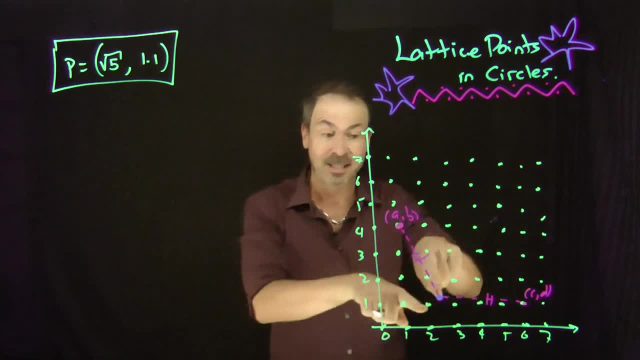 here. So if I want this distance, the hypotenuse is a right triangle. So Pythagoras says: oh, the distance squared is just the difference. It's the difference of the x-value squared plus the difference of the y-value squared. 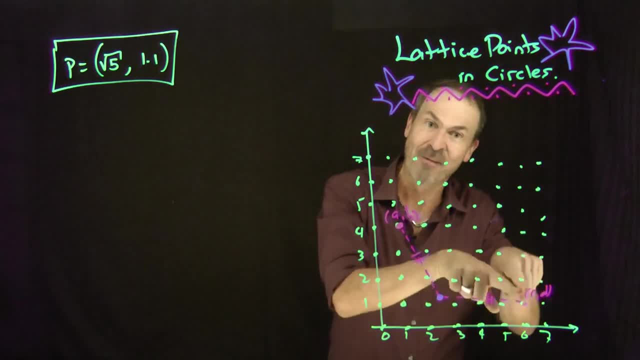 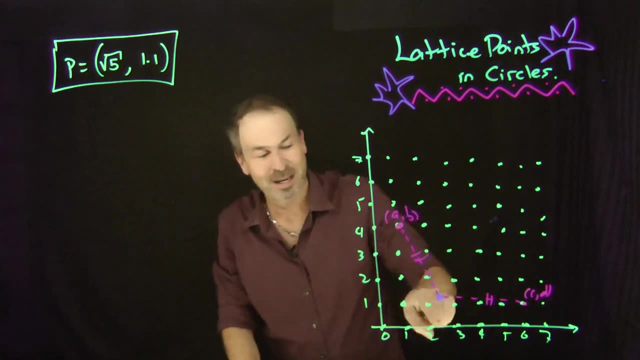 The distance here squared will be the difference of the x-value squared plus the difference of the y-value squared. I want the same distances. I want the same distances squared. Therefore, I want the difference of the x-value squared plus the difference of the y-value squared. 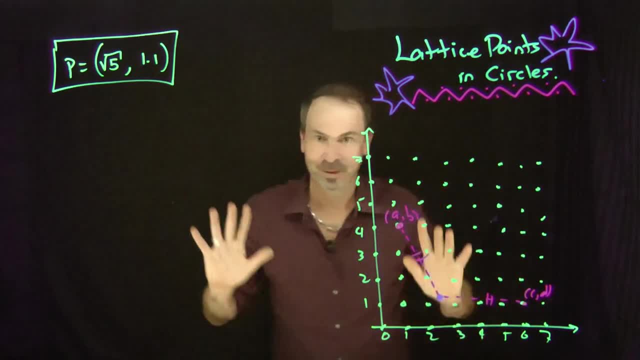 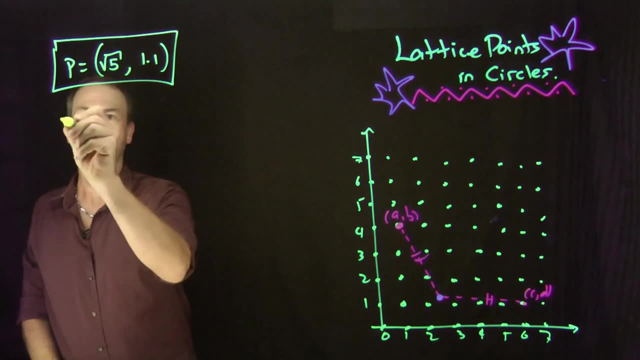 to equal the difference of the x-value squared the difference of the y-value squared over yonder. Okay, Let's translate into algebra What's going on. So I want this difference of x plus this difference of y, each squared. What's it going to be? It's going to be a. 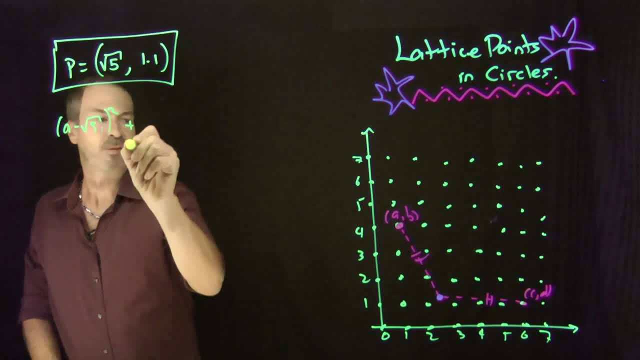 minus root, 5 squared plus the difference of the y-values. b minus root 5 squared plus the difference of the y-values. So I want this difference of x plus this difference of b minus 1.1 squared. If this picture were happening, we'd have to equal c minus root 5. 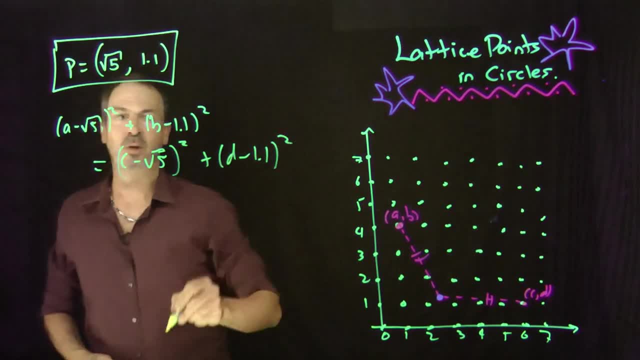 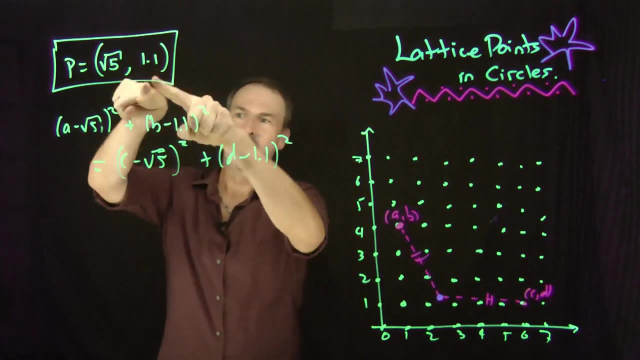 all squared plus d, minus 1.1, all squared. Alright. now remember: a, b, c, d. a, b, c, d are whole numbers. 1.1 is a very nice rational number. It's a fraction. It's 11 tenths. 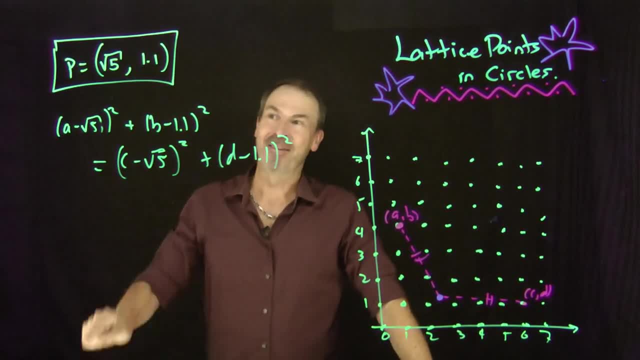 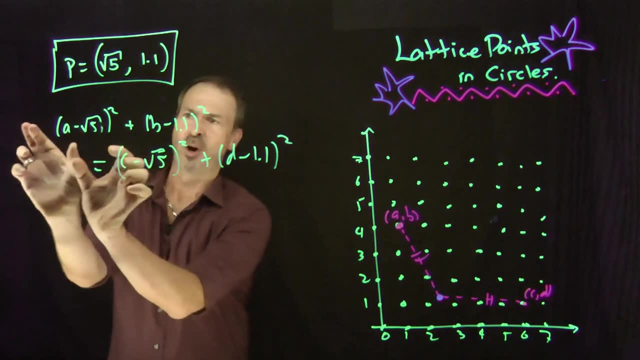 And I've got this root 5, which we know is not a fraction. So I have a feeling the irrationality of root 5 is going to be a key play in this game here. Alright, if I'm going to focus on root 5, let me bring all this root 5 stuff over to one side. 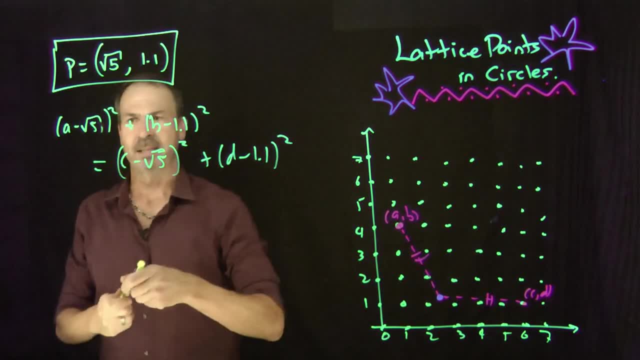 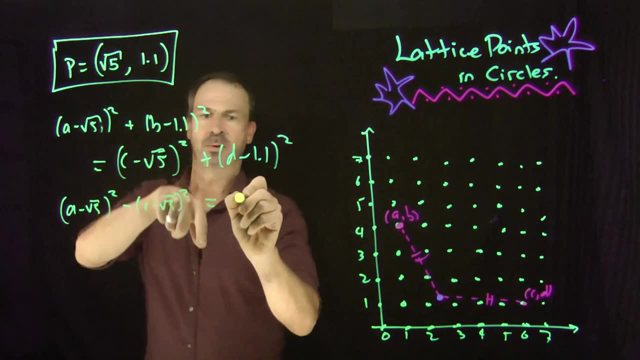 Let me subtract c minus root 5 squared from both sides and bring this over to the other side. So this is really a minus root 5 squared minus c minus root 5 squared equals d minus 1.1 squared minus b minus 1.1 squared. 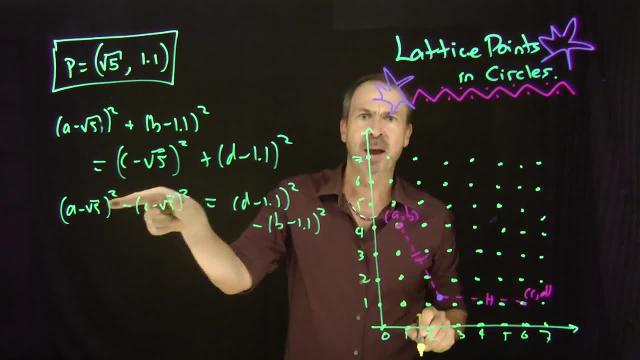 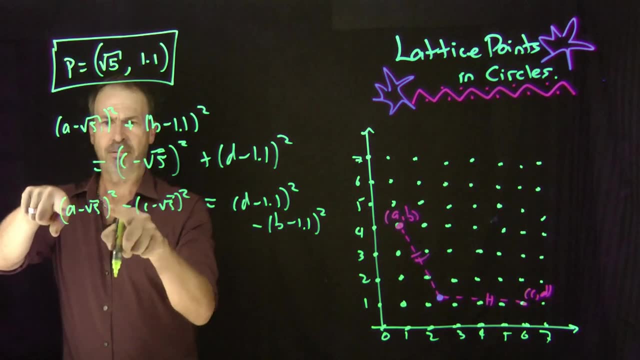 In fact, let me try to pull out that root 5 from this, indeed, So let me expand the brackets here. I'll leave this right-hand side stuff the same. Don't do any extra work unless you have to. a squared plus 5, a squared plus 5 minus 2a root 5. 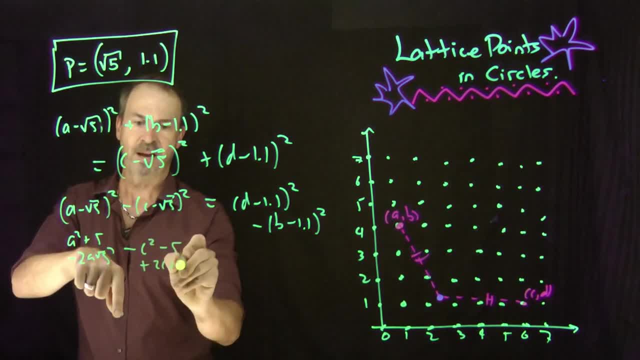 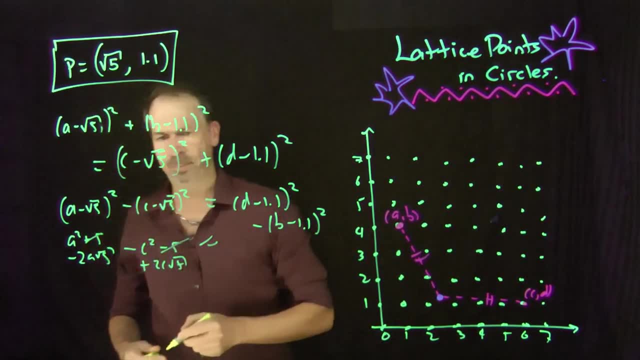 minus c squared. minus 5 plus 2c root 5 equals this stuff. Okay, how's that for a bad board technique? Plus 5 minus 5.. Okay, it's a little bit simpler, Okay. so now I've got an a squared and c squared here, minus c squared. 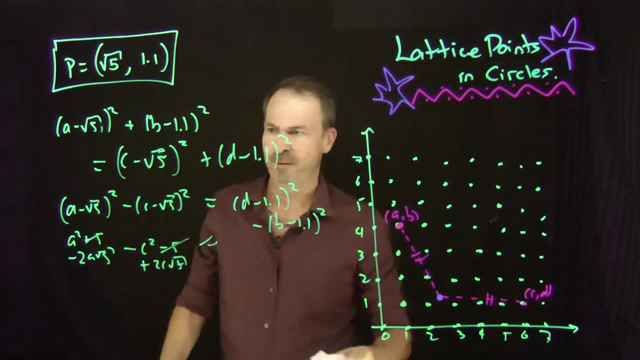 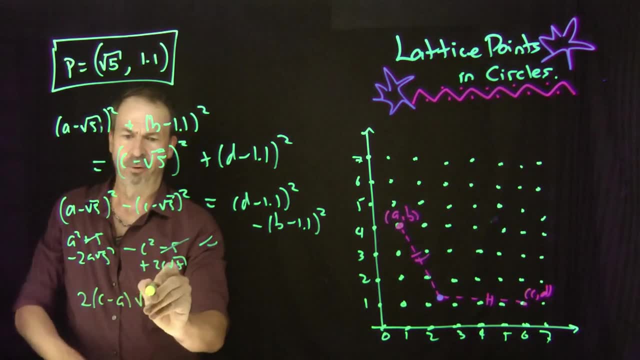 Let me bring that over here and just keep, really keep, all the root 5 stuff on the left-hand side. So messy technique. Oh no, I'll do it here. What's it gonna be? 2c minus a root 5 would equal. 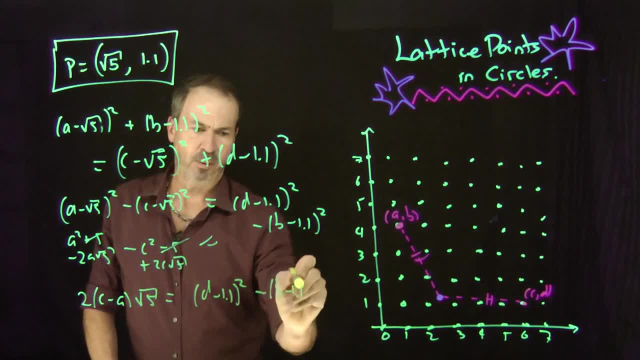 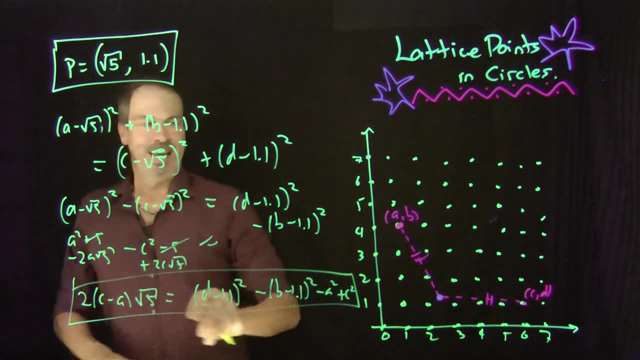 d minus 1.1 squared, minus b minus 1.1 squared, Bring the a squared over and bring the negative c squared over. So right now, if this is happening, then that's the algebra that's happening, All right. all right, so we got that equation, is that? 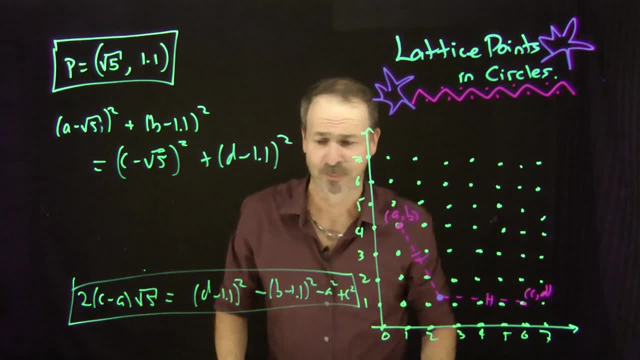 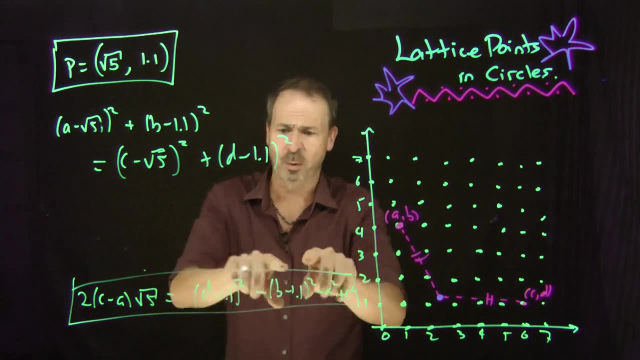 Now this is trouble, troublesome. This is potentially troublesome because, because this is integer, integer, integer, integer, integer, 1.1 squared, 1.1 squared. Everything here is a rational number. It's a nice rational number, It's like one, it's a finite decimal. 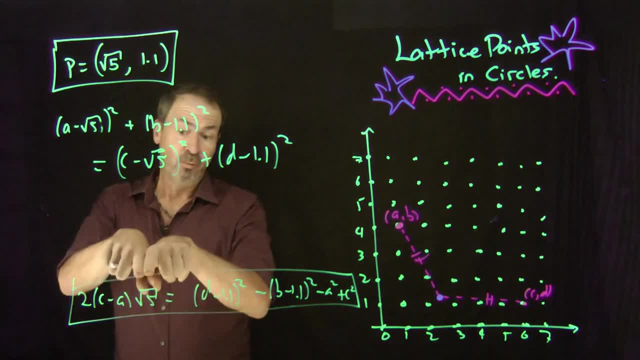 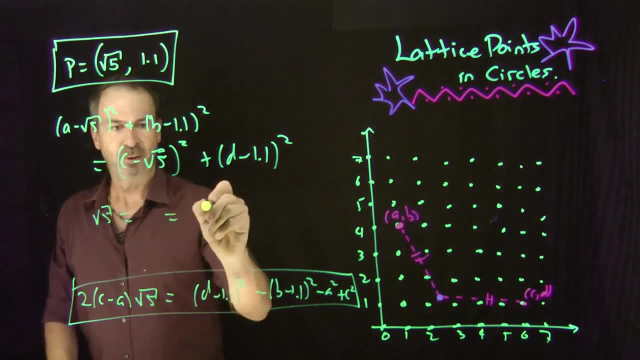 Over here I've got 2 times an integer. Root 5 times an integer equals a rational number, So I could then argue that root 5 would be all this stuff, which I'm not gonna bother writing again, divided by 2 times c minus a. 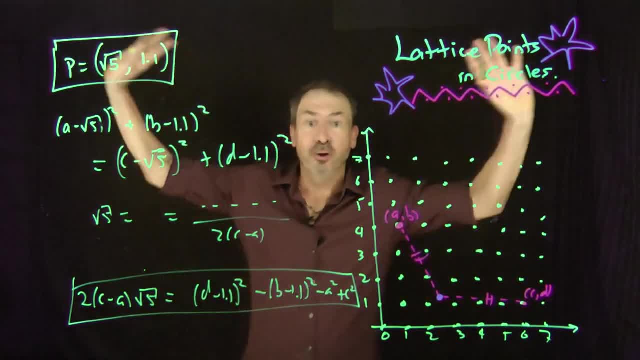 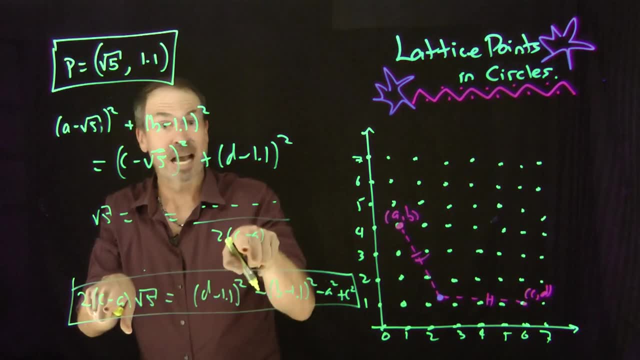 which will then tell me that root 5 is actually a rational number. Not true, not true. You see, there's one way out of this pickle. It may be that this is 0, which means I can't divide on both sides. So for this equation to be true, knowing that root 5 is a rational 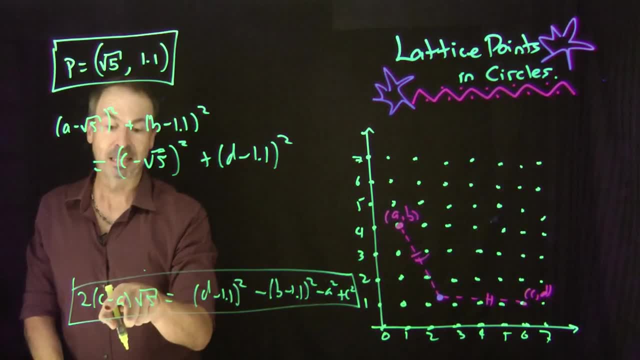 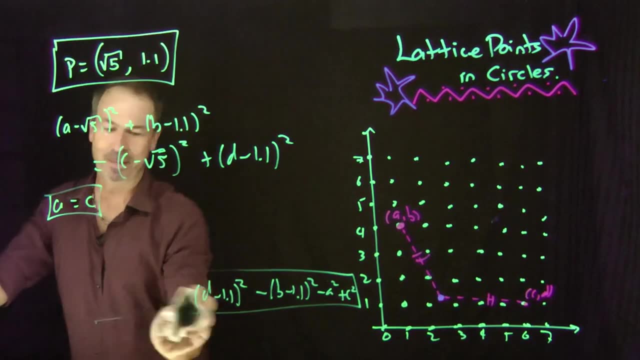 I am forced to conclude that this number here is 0.. c minus a is 0. That is, I'm forced to conclude that a and c must be the same number. All right, all right, great. a and c must be the same number. 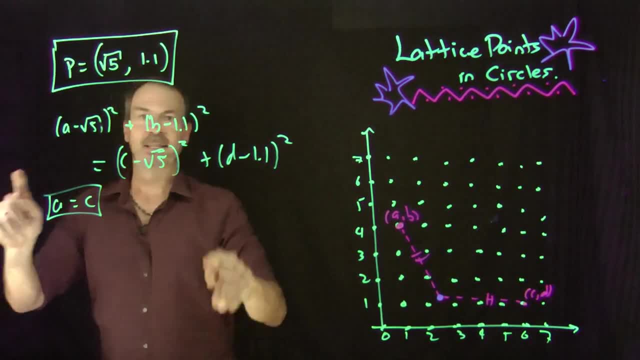 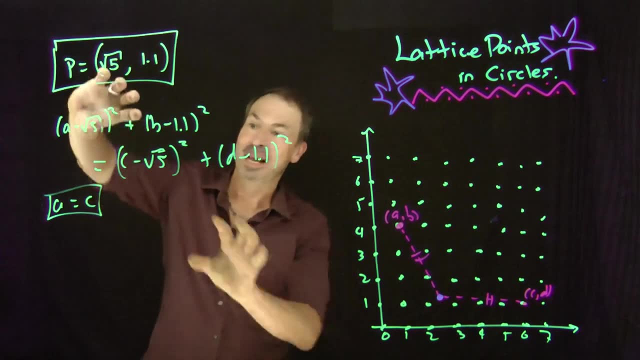 So the algebra tells me that a and c are the same value. So actually my picture's off doesn't matter, because I'm playing this equation now- a minus root 5 squared here, a minus root 5 squared here, they're the same value. So my equation really now boils down to: 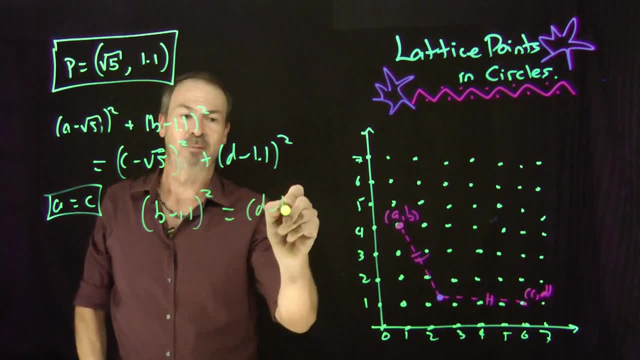 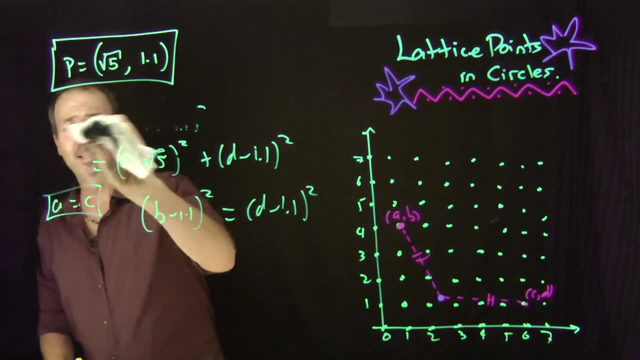 b minus 1.1 squared equals d minus 1.1 squared. All right, okay, let's keep going. Let's keep going. This is fun. So if those two distances are equal, I must have that a equals c and this next relationship holds. 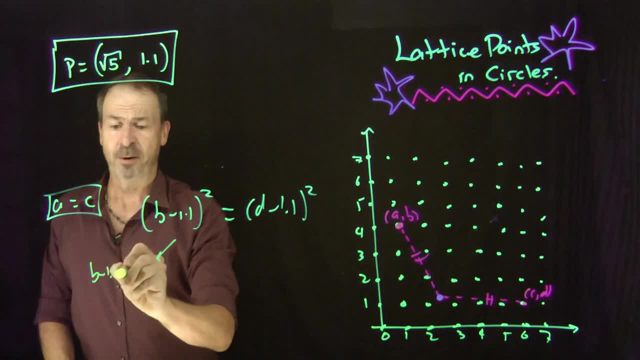 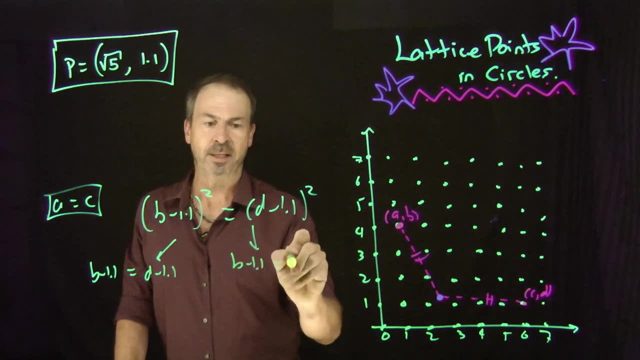 Something squared equals something squared, so that I could be the same thing. b minus 1.1 equals d minus 1.1, or one's the negative of the other. b minus 1.1 equals negative d minus 1.1, so it's 1.1 minus d. 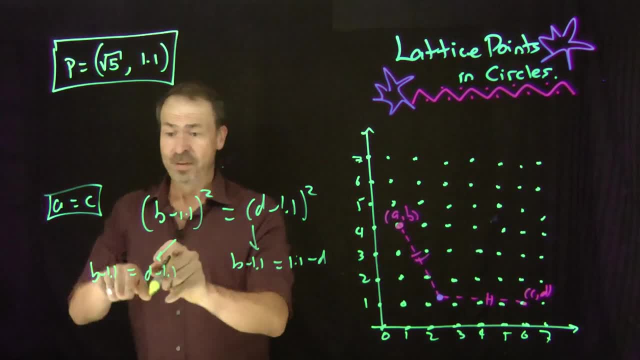 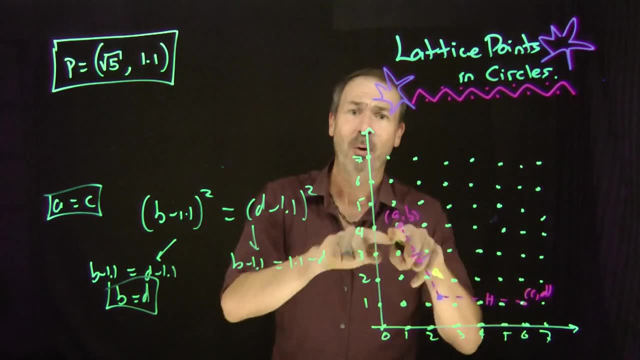 All right. what are the consequences of that? Oh, this tells me that b equals d, b equals d. Oh, so a equals c and b equals d. Oh, maybe they're at the same point to begin with. Well, that's not happening. That's not happening. 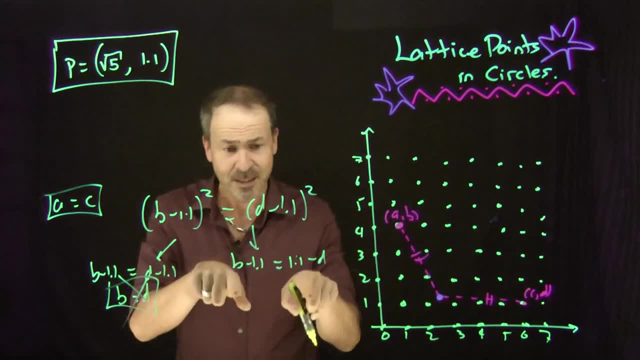 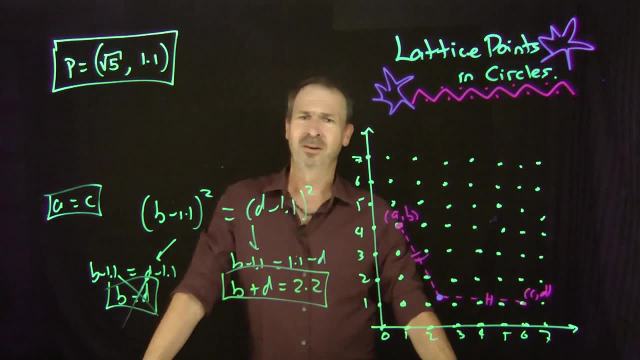 I definitely want to consider separate points, In which case this must be the case which tells me that b plus d is 2.2.. Can that happen? Huh, so now we're boiled down. If these two distances are the same, 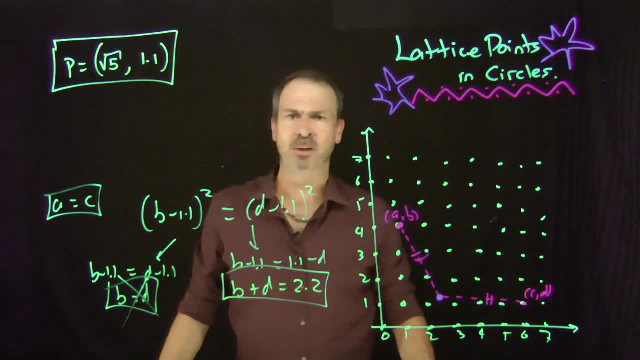 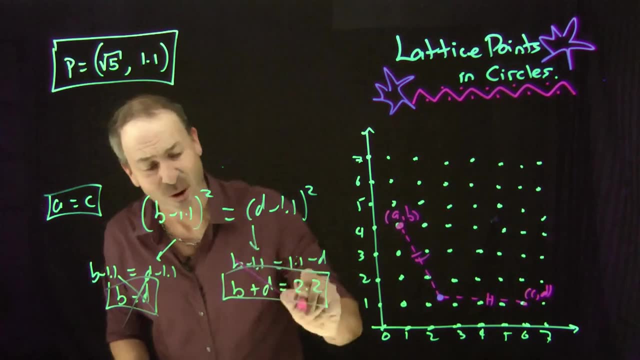 I must have the x-quadrants being the same and b plus d adding up to 2.2. But b and d are whole numbers and two whole numbers do not add up to 2.2. Which means that's not happening. That's not happening. 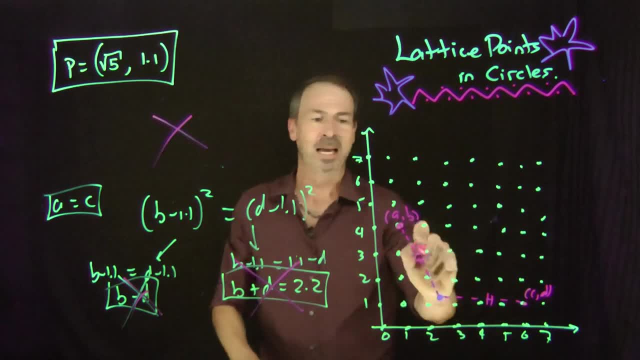 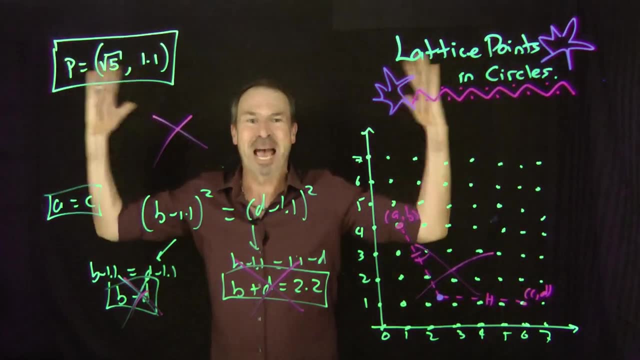 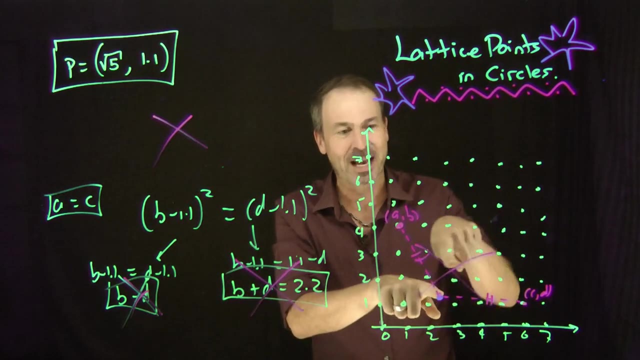 Which means the original equation is not happening, Which means this picture is not happening. You cannot get two lattice points the same distance from that special point p right there. Which does it, Which absolutely does it. I think that is amazing. We can actually pinpoint one Literally. there's one, all of whose distances from different lattice points are different values. 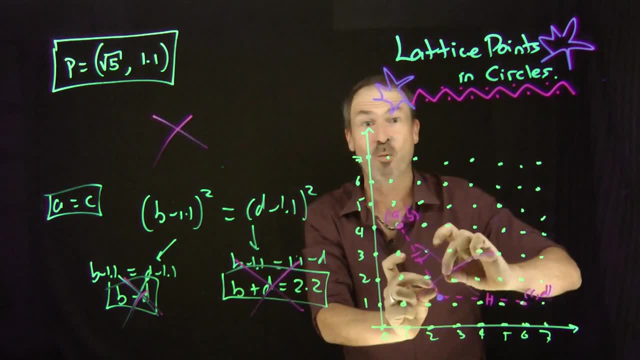 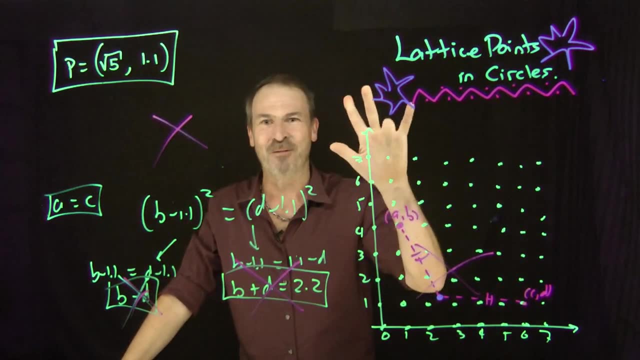 That's amazing. In which case, just expand circles, Hit them one at a time, boop, boop, boop, boop, boop. got a little bit bigger and you'll get circles that contain 0,, 1,, 2,, 3,, 4,, 5,, 6,, 7, all the way through all the counting numbers on their interiors. 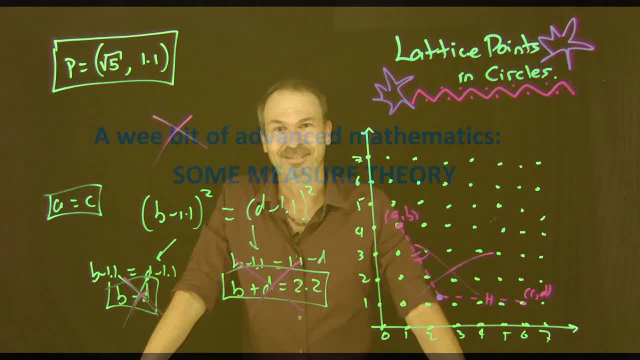 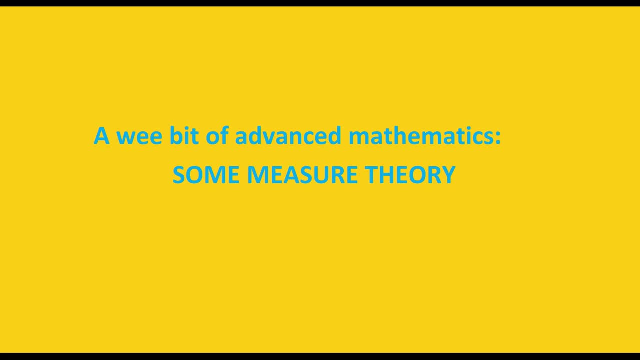 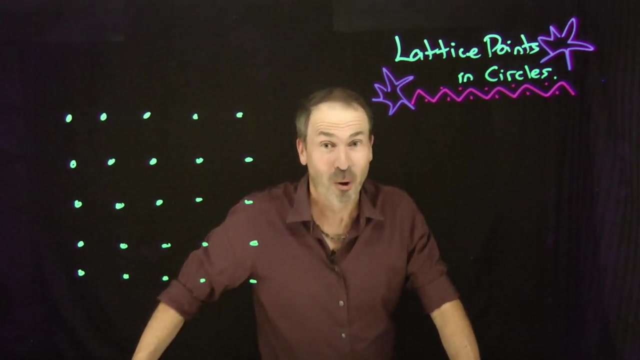 That's amazing. I love it. If you've done some undergraduate mathematics or graduate school mathematics and measures theory, we can actually prove that almost all points in the plane have this magic property of having distinct distances to all the lattice points in the plane. 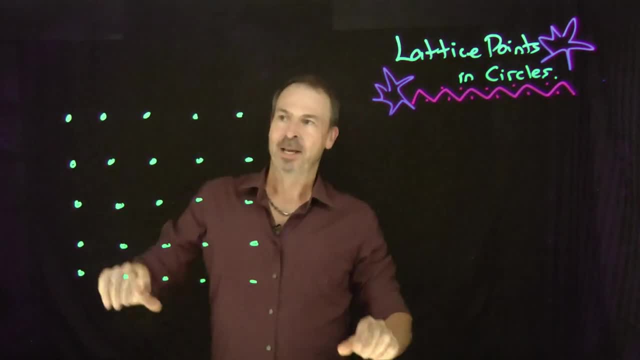 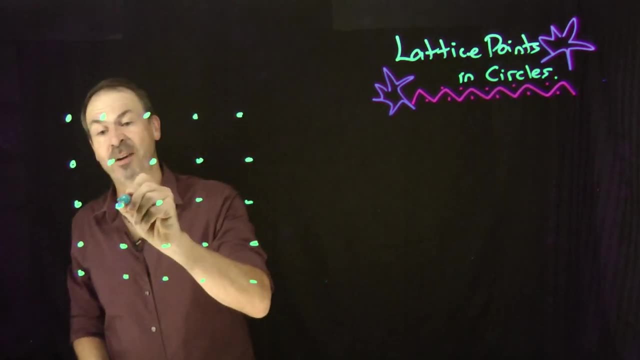 Whoa, Here goes. Here's why. Here's why, First of all, there's definitely a countable number of points, lattice points in the plane. Okay, countable number of points. In fact, there's a countable number of pairs of points. 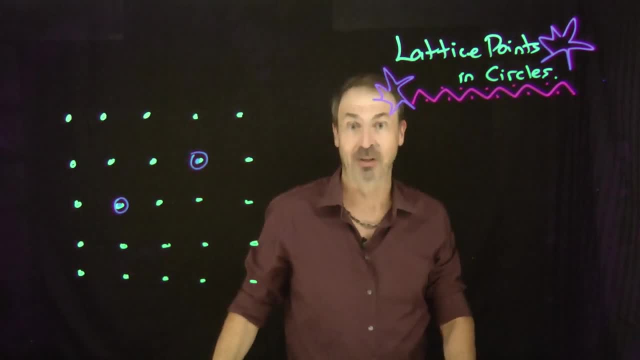 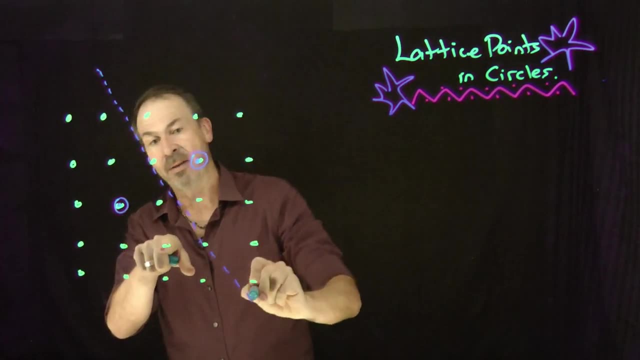 If I just choose a pair of points, there's countably many pairs I can choose. Great, For each pair of points there's a line of equidistance. These are all the points that are equidistance from those two lattice points.